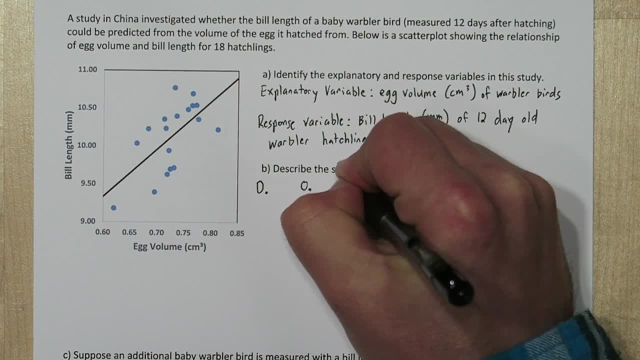 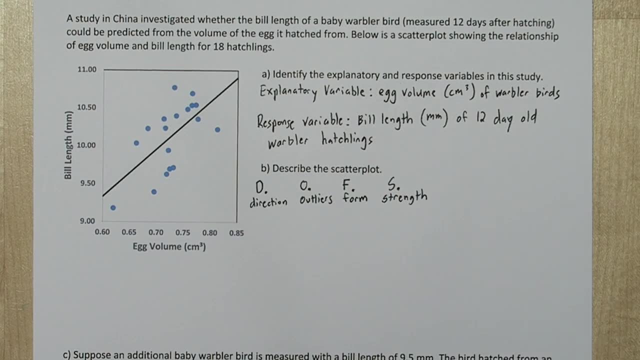 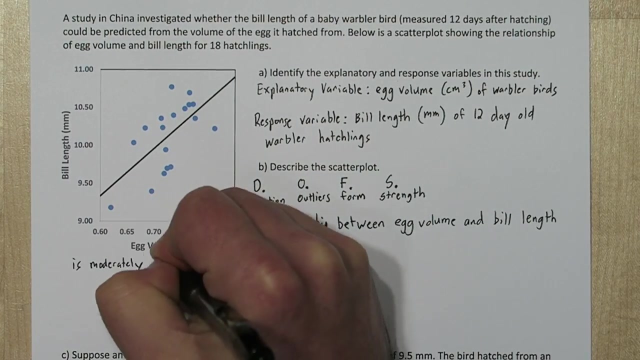 There's four things you need to talk about when you describe a scatterplot. The acronym DOOFS might help. You need to talk about the direction, outliers, form and the strength. So we'll say the relationship between egg volume and bill length is moderately strong, positive and a linear relationship. 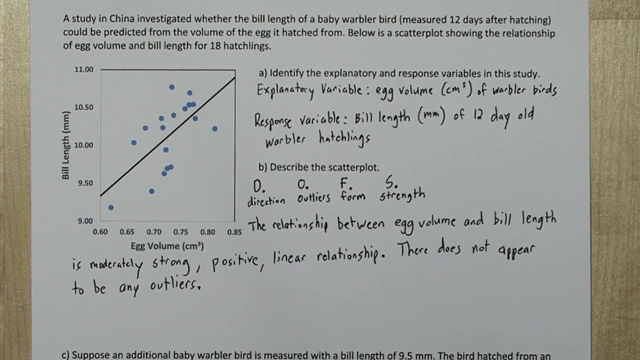 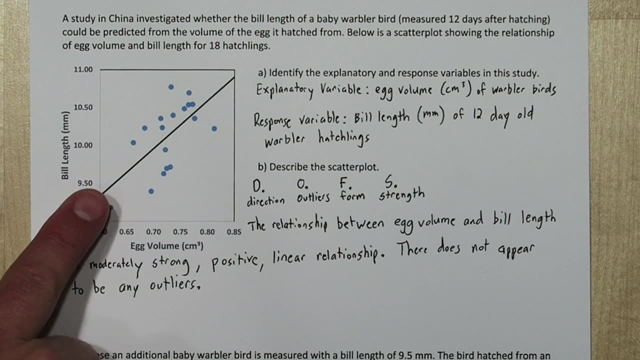 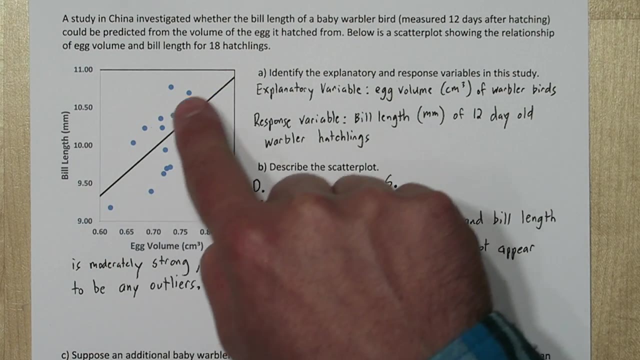 There does not appear to be any outliers. So we know it's moderately strong because most of our points are fairly close to our model line here. It's positive because as egg volume increases, so does bill length. It's a linear relationship, because that's the form that seems to describe this scatterplot best. 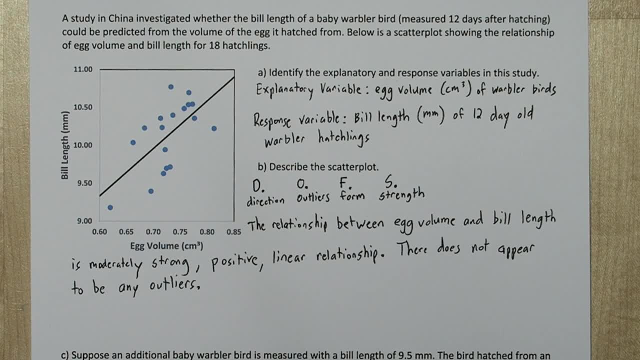 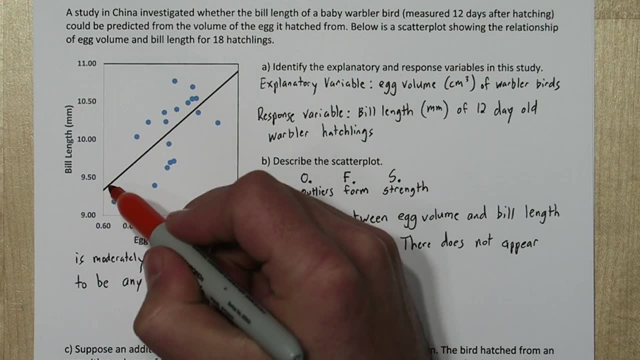 And there's no outliers, because nothing is terribly far from our model line. So we've described the scatterplot. Now, if this additional bird has a bill length of 9.5 millimeters, that's right here, and it has an egg volume of 0.83,. 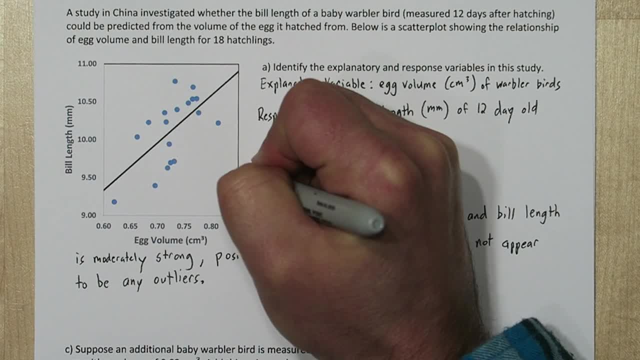 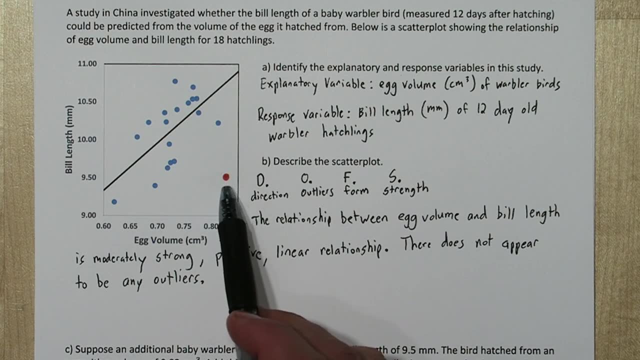 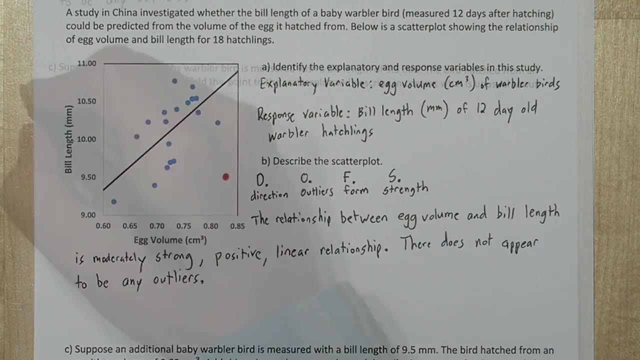 that's probably a point about right here. Now notice this point is pretty far from our model line. Typically we'd expect a bird with an egg volume of 0.83 to have a bill length much closer to about 10.75 millimeters. 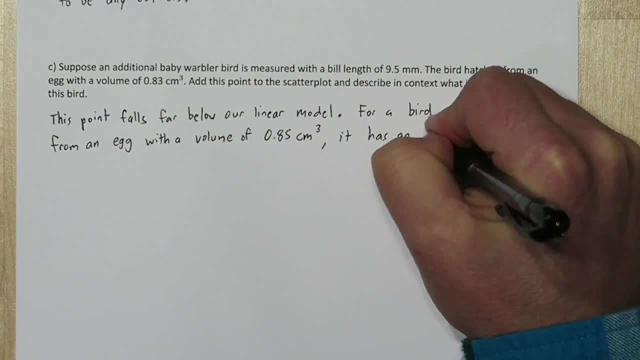 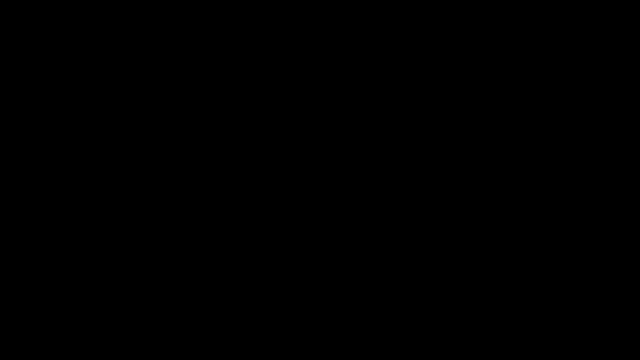 So this particular bird has an unusually short bill length relative to its egg volume. If you liked this video and want to learn more about scatterplots, least squares, regression residuals and how to use your calculator, check out this playlist. Lots of students have found the first video on the playlist particularly helpful. 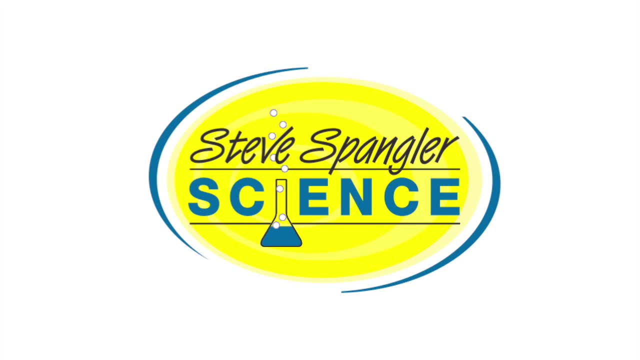 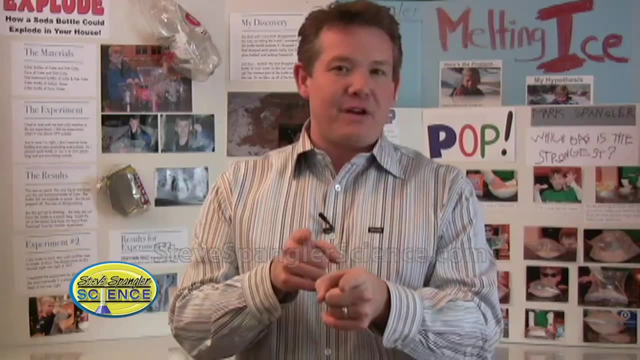 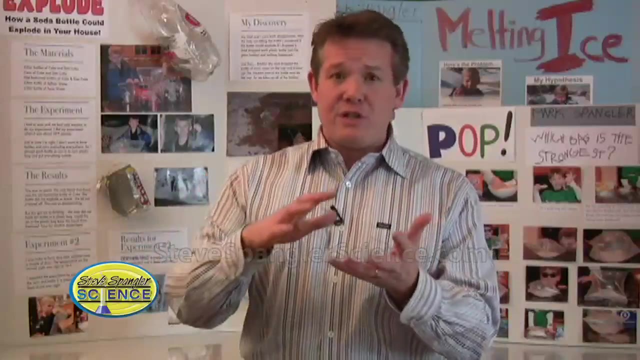 I'm Steve Spangler and I'll bet you're looking for a science fair project. you've come to the right place here for the science fair page here at stevespanglersciencecom. Now you might just be looking for those petri dishes and the auger, and you know exactly. 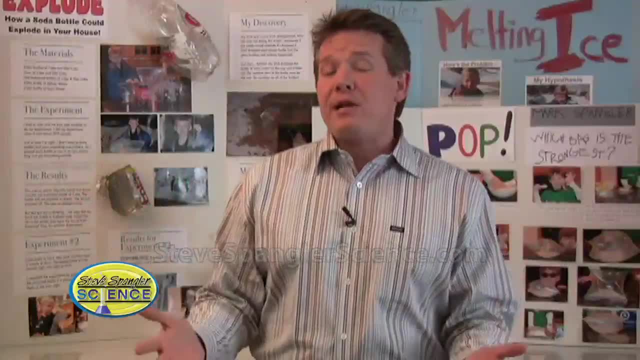 what you're going to do with your project and of course, we'll help you out that way. but we put this page together for those people who are also looking for some ideas, because you might have noticed on our site, if you look at the navigation up above, that not only